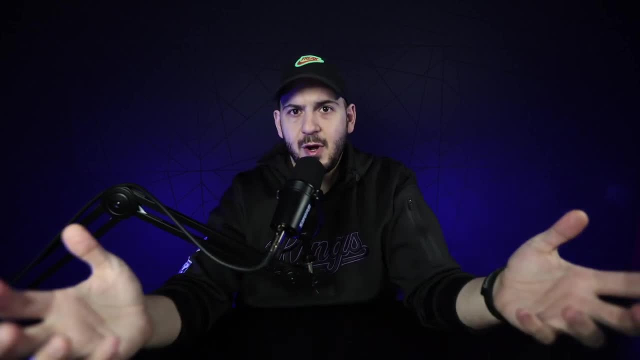 video. you got to do me a favor. drop me a comment, Let me know if you're a part of the five-week program. You can just drop a comment that says 5WP- five-week program, and that will let me know. 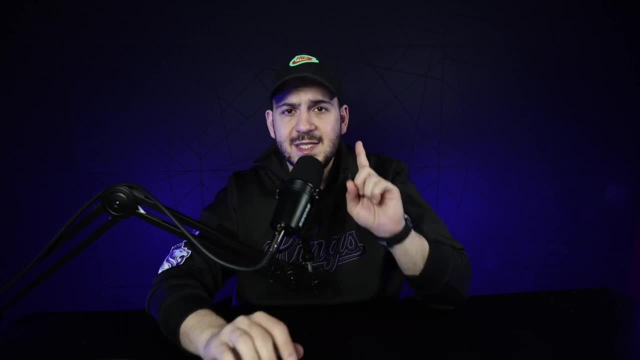 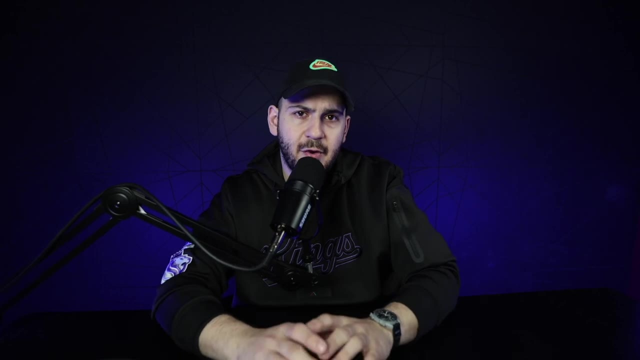 how many of you guys are actually participating. And if you haven't done it already, it's never too late and you still have time. Go down below into the description. click on that Discord link, come join us and let me help you find your first vulnerability. But before we jump into our lab, 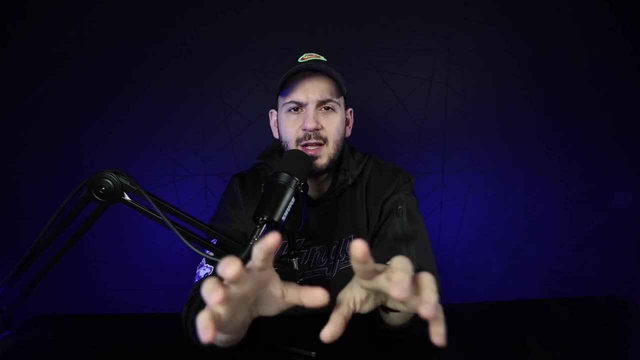 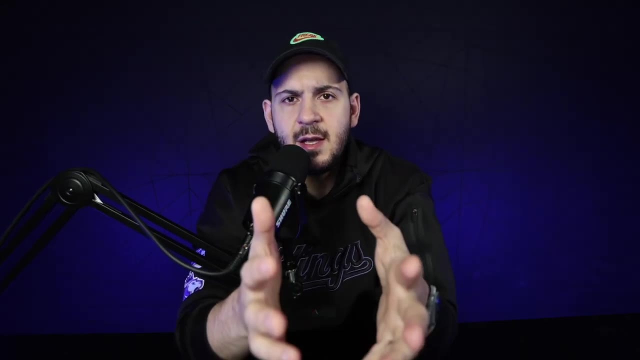 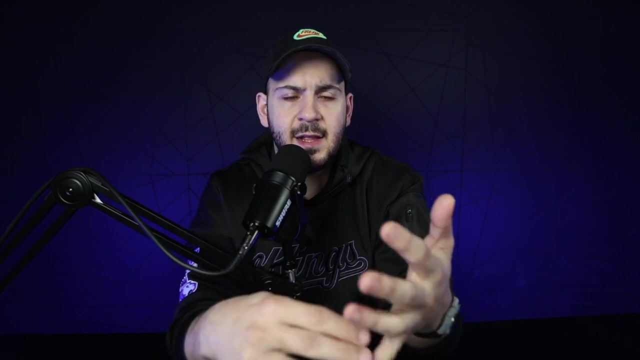 let me explain what CSRF is. I'm going to show you what an example of a good versus bad CSRF looks like, and we're going to solve some of our labs. For CSRF specifically. it pretty much means that an attacker can force their target into an unwanted action. That action could be things like deleting their address. 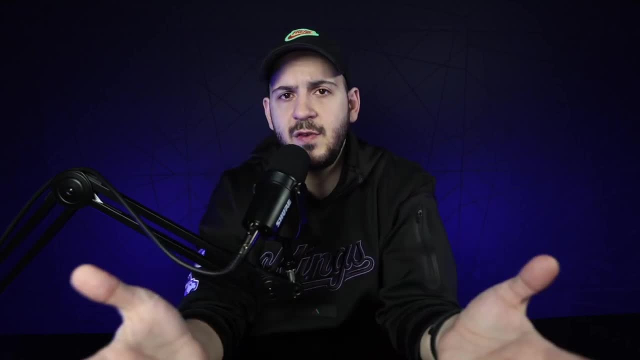 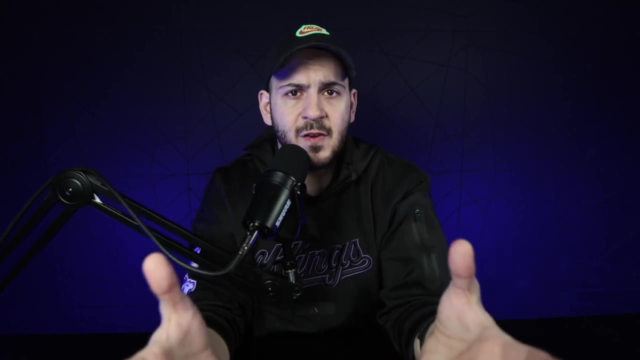 changing their name, changing their username or even turning off the notifications, which in some cases that is not really a higher priority vulnerability, And that is an example of a bad CSRF, because you want to be able to justify the criticality of your CSRF by 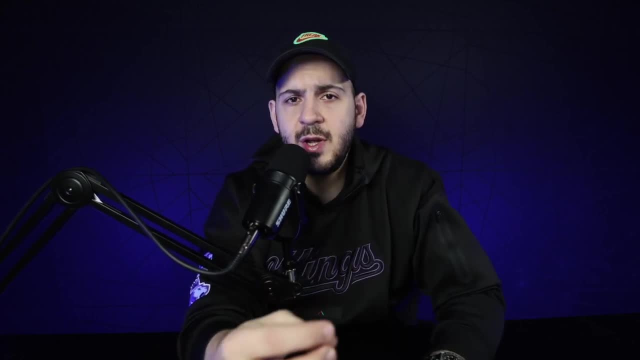 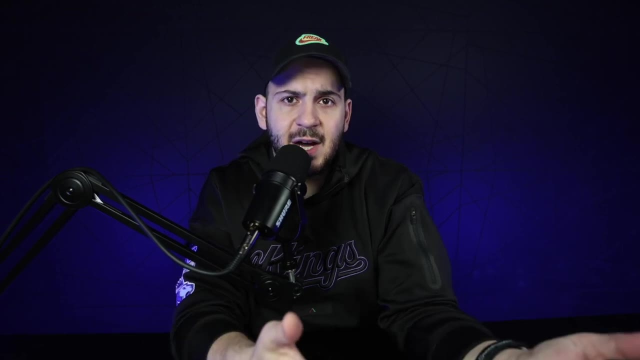 answering the question of: so what? How is this going to affect that user if I force them into this unwanted action? So, for example, if you force them into changing their password, obviously you can gain access to their account and they're going to lose access to it, versus turning off. 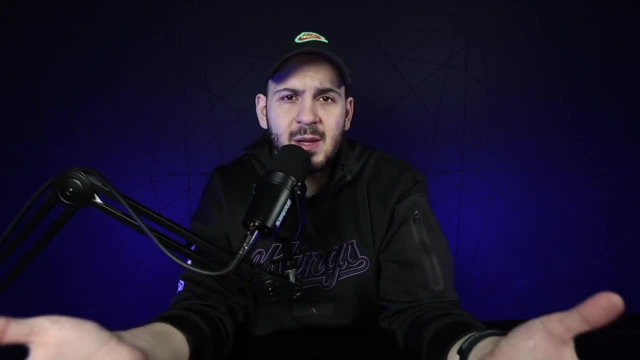 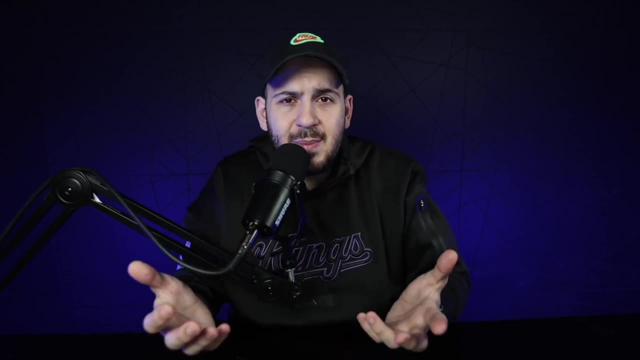 notifications, which isn't really a critical vulnerability, but in some cases it is still valid and some companies are going to actually award it, But in this case, I think it's maybe a low or medium at its highest value And a lot of times companies aren't going to actually 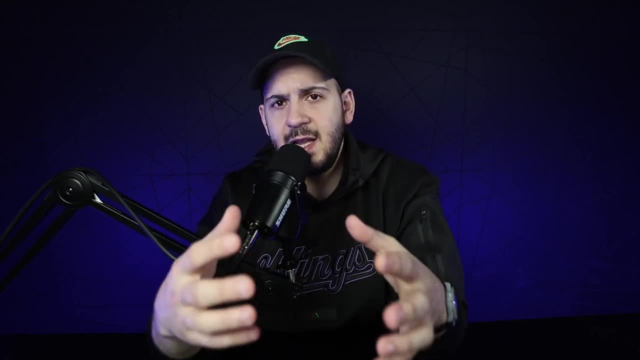 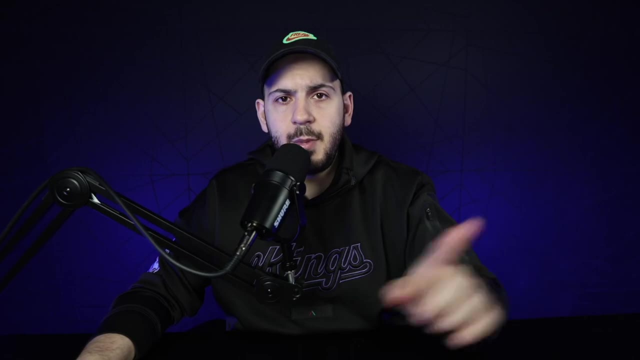 acknowledge it. So keep that in mind And I'll see you in the next video. Again, it is just dependent on what the action is. but there are also other ways you can bypass CSRF mechanism, which I will show you in this video. But for now let's jump into 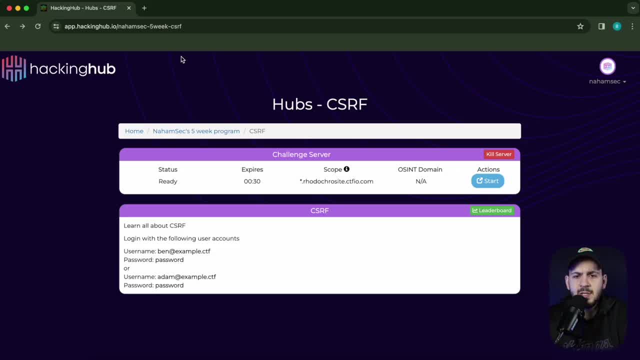 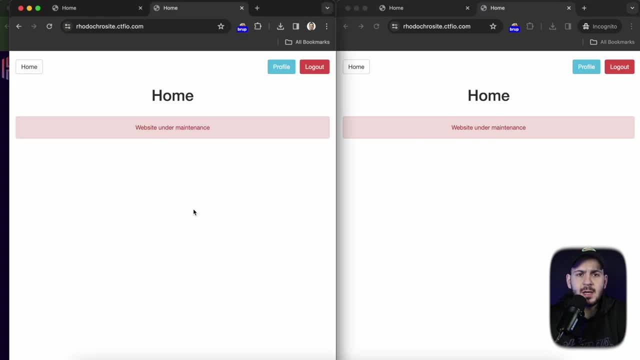 our lab. We're going to go to hackingupio. If you want to follow along, go to this hub. It's under my five-week program hub. click on CSRF and launch it And it's going to give you a username and password And, as you can see, I'm already logged in here and we're 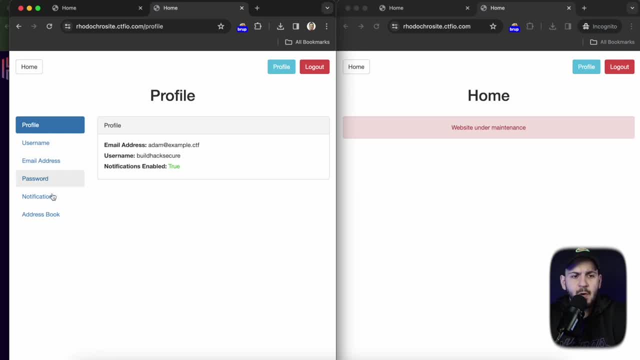 going to take a look at what functionalities are within the profile page here. So, for example, in this case, like I mentioned, there's notifications here And if I pull up Kaido and intercept this, we can see that it's sending this request. 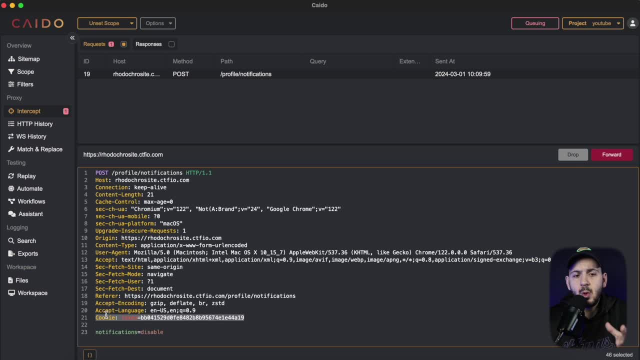 and it's sending it to profiles notifications, And the only header that we see here is a cookie header. Everything else here is for the browser And it's sending this post header notification and making it disable. So in this case, we don't even see a single hint. 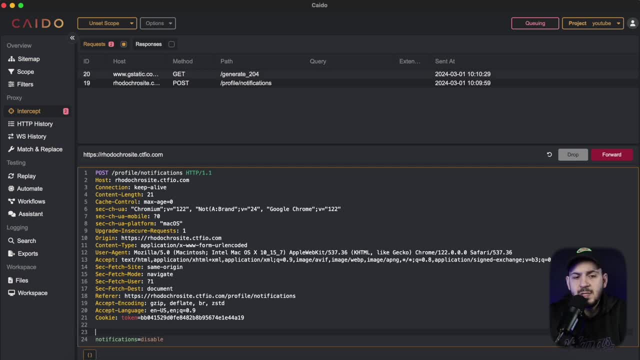 of a CSRF protection, because usually you would see something in the headers, for example, that will have XCSRF token And it has some values where sometimes you will see it at the top of the page, but it's always terrible in the lower left corner of the page because 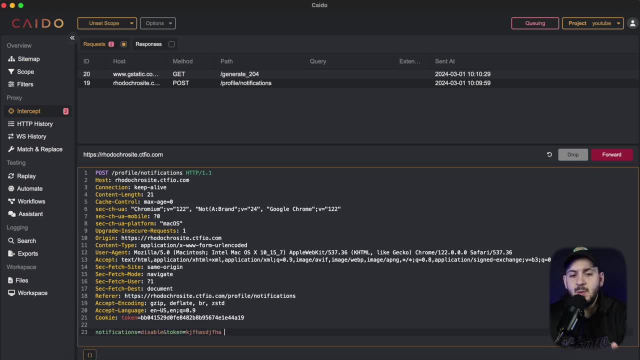 it doesn't create a complete text, So that's something that you can easily do on the browser. I'm just going to do this and we'll. I'm going to take the next step. It's called theagramco, which is a name for a CSS YouTube video. It's not going to be. 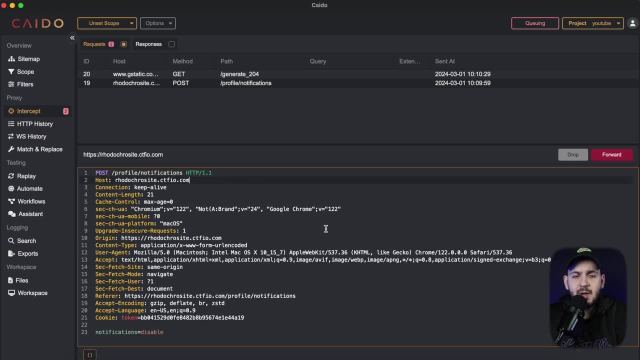 a very long video, but I'm going to tell you a little bit about the program. It's a YouTube video. You will see that it's going to be here in the lower right corner of the page, but it's going to be free. I think you can also see that the name of'em'. 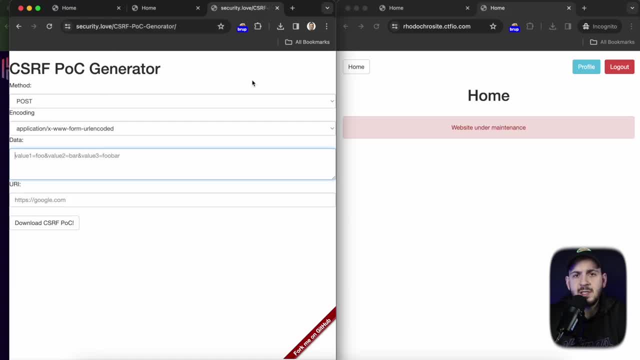 being the name of'em' is a CSS videos, So that's the name of my video, So it's going to be free. If you're interested in this, I can put this in the chat. if you want, I'm can actually go into here. to securitylove csrf poc generator. give them the data and it will create. 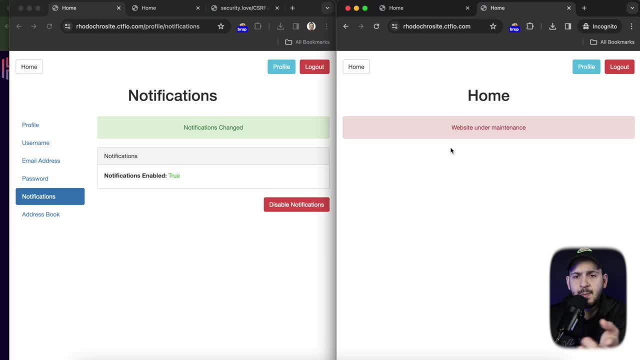 that poc for you and once your target, for example, on the right, if the right browser clicks that link that is created by the csrf poc, then it would immediately disable the notifications. so now let's take a look at this example and, as you can see, notifications here are enabled and i have my 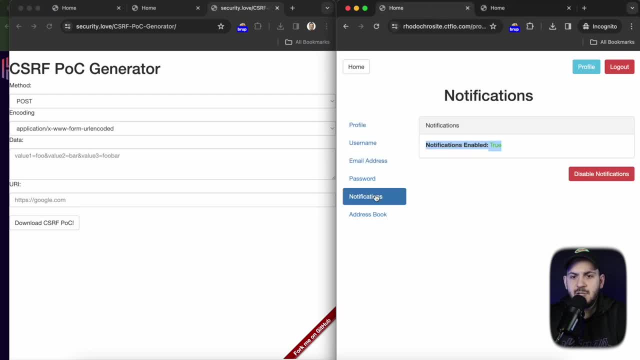 csrf poc here. we're going to click on this button and we're going to refresh this page. as you can see, it says notifications change and it turns out that we were able to turn this into false. but again, please keep in mind this isn't really a critical vulnerability. disabling notifications isn't a. 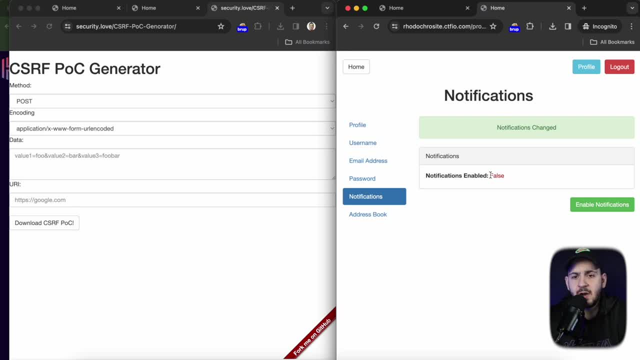 vulnerability, but i want to show you an example of an action that has no csrf protection against it, and this is a good case to take a look at. let's look at other functionalities here. let's go to password. this case, changing password is going to be kind of hard because even if there isn't a csrf, 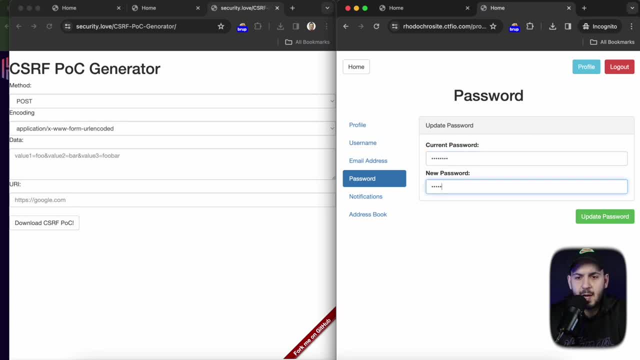 protection. for this it requires the current password. but i'm going to try it one more time and i'm going to. you can see that it's not going to change the password. it's going to change the password and i'm going to try it one more time. and i'm going to try it one more time and i'm going to. 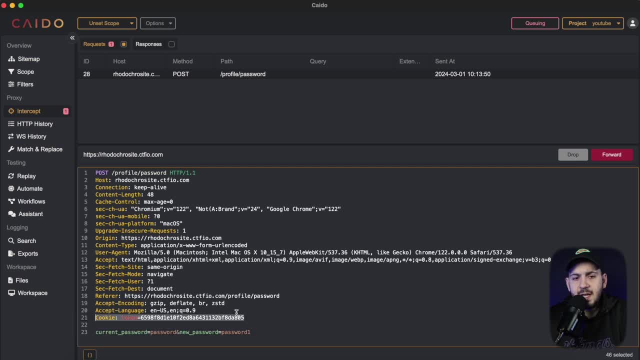 request this. it's going to send this request and you can see again. there isn't any csrf protection here. but even though there isn't one, the current password itself kind of acts as a mechanism here that stops you from reporting it. so in some cases some companies may take this. i personally would. 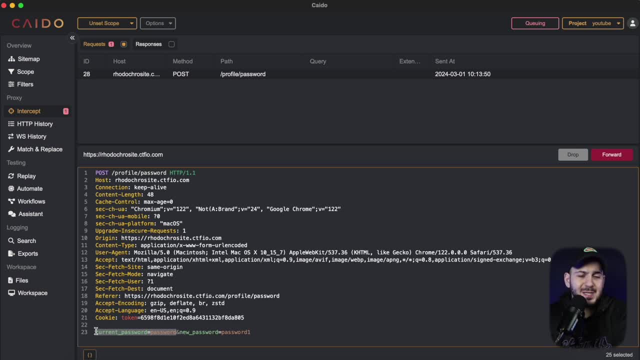 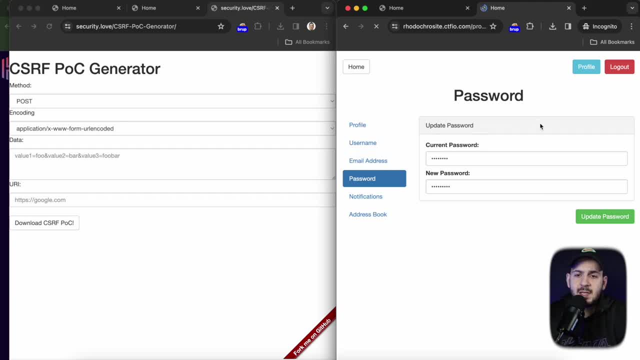 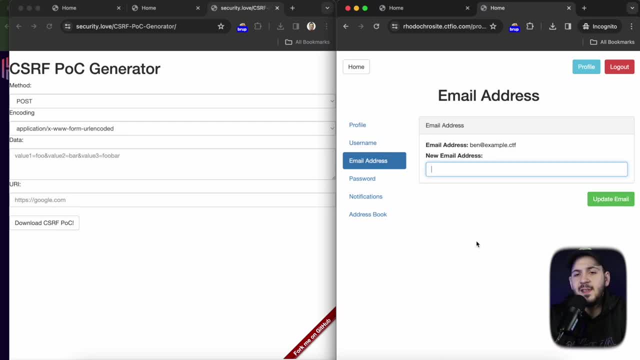 things. this is actually a really good place to look for csrf. anything that allows you to alter a user's information that could gain you access to their account is always a good place to look at. so, for example, in this case we have the email address. sometimes you may be able to. 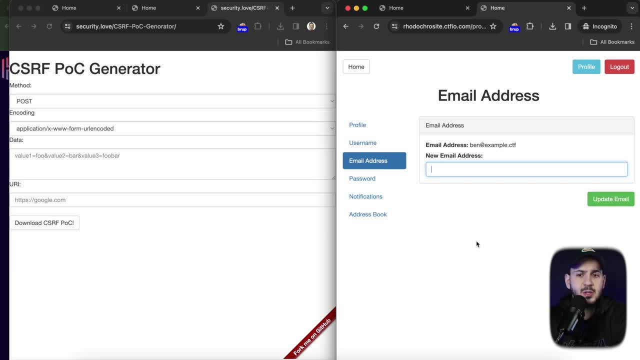 actually delete or add a api token, for example, if it allows you to put your own api token. sometimes you can add a new secondary email address or add yourself to an organization. those are all actions that are very sensitive. so in this case, if we update this, i'm going to update. 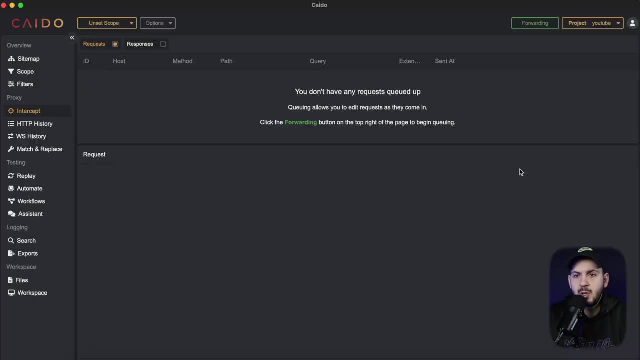 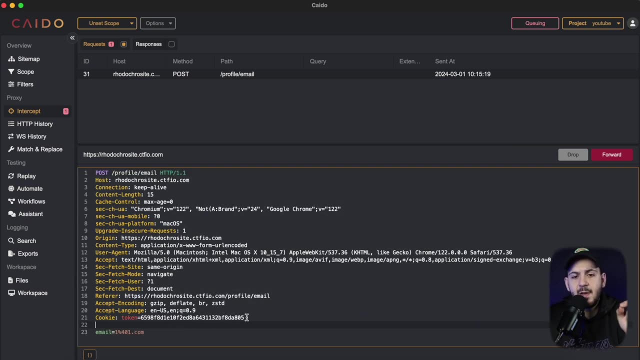 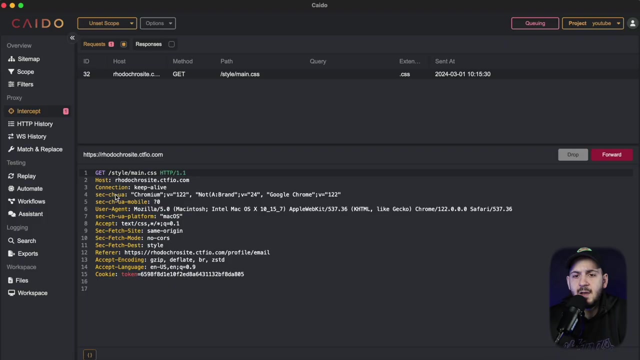 this to one at onecom. i'm going to make sure we're intercepting this. i'm going to update this. we can see that is the same thing here, same thing as last time. there is no csrf token here, but this is a great example of a good csrf to report because, at the end of the day, if you change that, 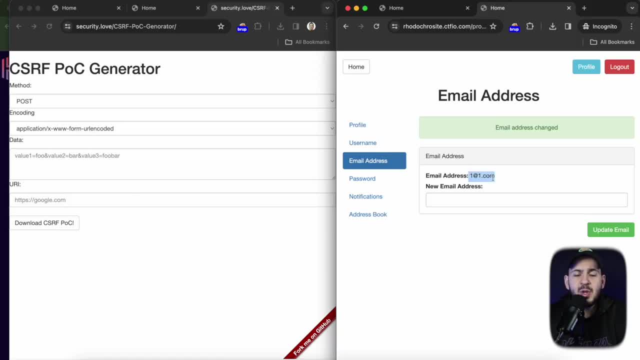 email address and it's becoming one at onecom, you actually fully have taken over an account and this is a good csrf, leading to account takeover, which in some cases could be a high or a critical, depending on the program and how the application is created. but in this case there's, and why this? 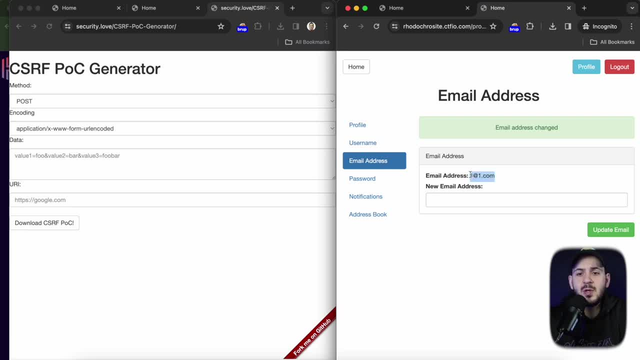 is valuable is because, by changing the email address, what we can do is we can take that email address, go to the login page, click forgot password and request a new token to send to our email address that we have changed to. so in this case you have a full account takeover. it may require 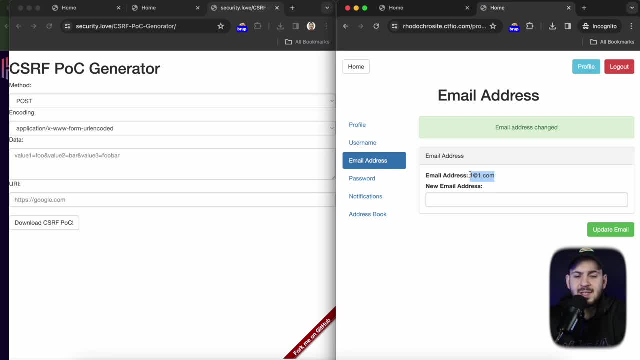 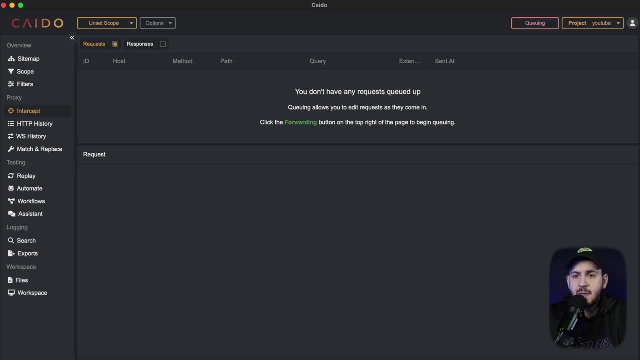 some user interaction. but again, this is a good csrf versus the bad csrf. in the case of notifications, there's going to be a lot of things that you can do to get a good csrf and you can do a lot of things sometimes where a functionality is going to present itself with a csrf token. so in this case, 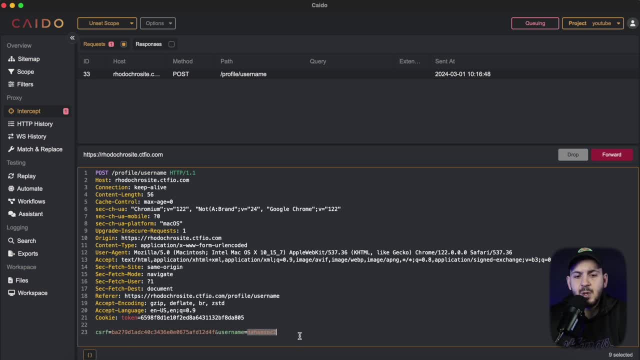 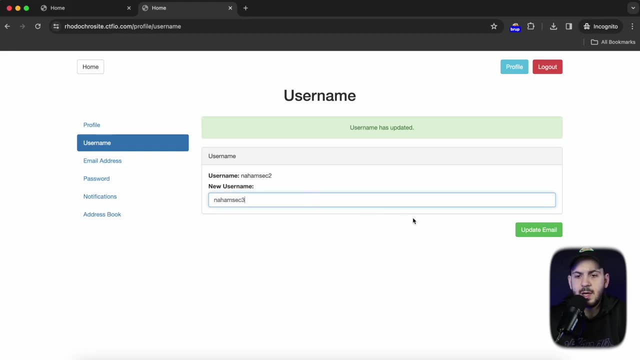 i'm assuming this one has something and you can see this has a csrf token and if we change the username and if you remove it sometimes or now, it works. we're going to try that one more time now. homestack three: we're going to update it when there is this value present for our request. what i 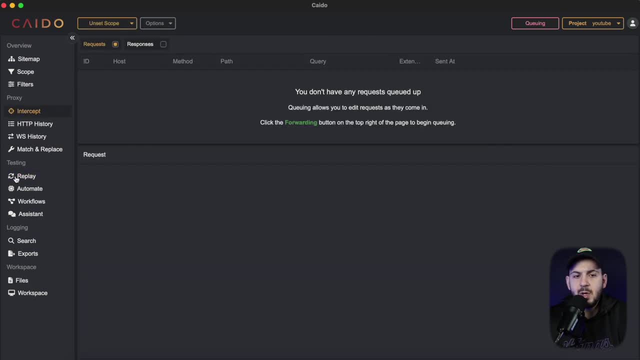 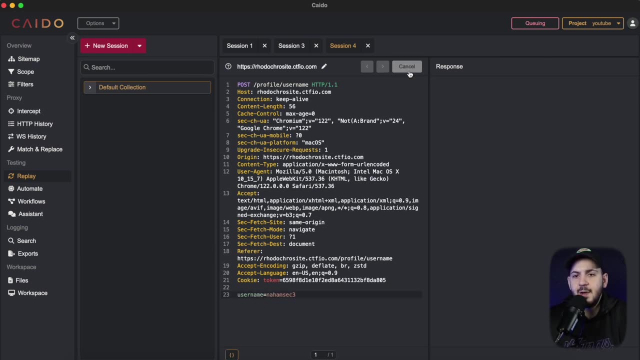 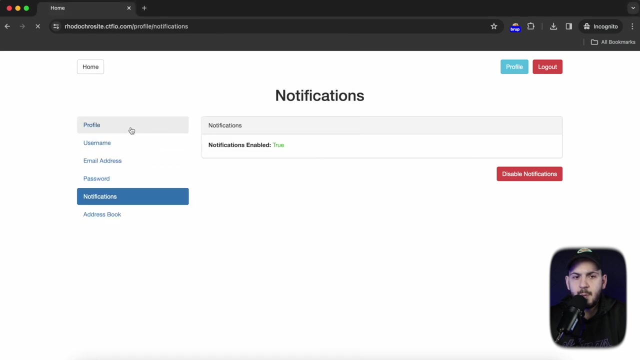 like to do a lot of times is i like to actually go into our repeater and see what i can do with it. can i remove this csrf parameter completely and see if it works? and if that does work, then sometimes it is a csrf on its own. i'm actually going to go and go to our profile again. let's make 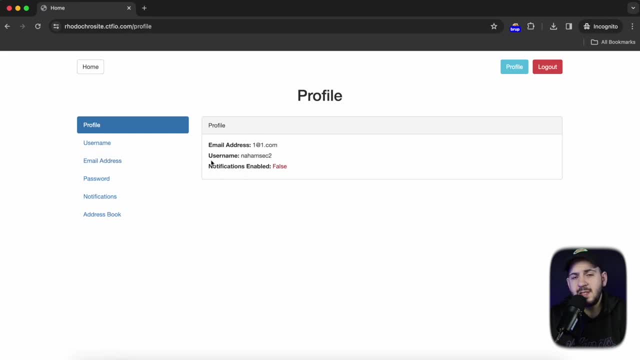 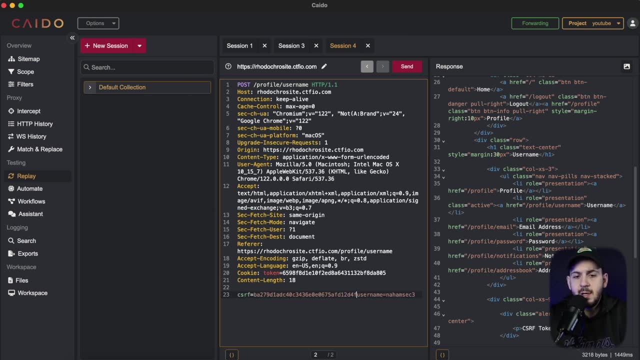 sure we're not intercepting. this one didn't work, but there's a couple other things that you can try. so the first thing when i see a csrf token is to completely remove it. the other option is to actually add a invalid token to it. so maybe if i change a value, it's just looking for a number of. 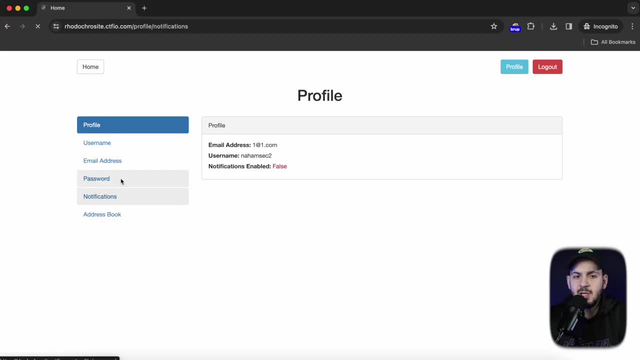 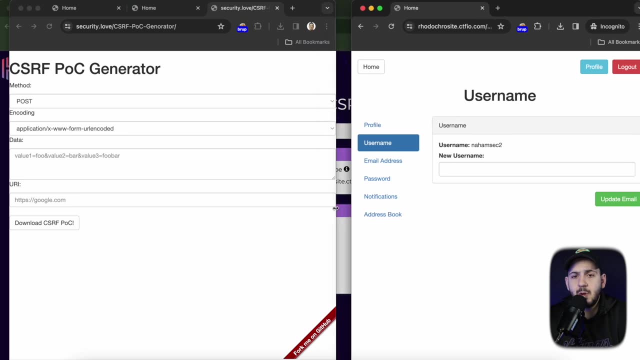 characters in that string. i see a csrf token and i'm going to go ahead and remove it and i'm going to send it. i refresh the page again. i go to username. that doesn't work. the third thing that i'd like to try here is, since we have the capability of making two different accounts, what i'm going to do is: 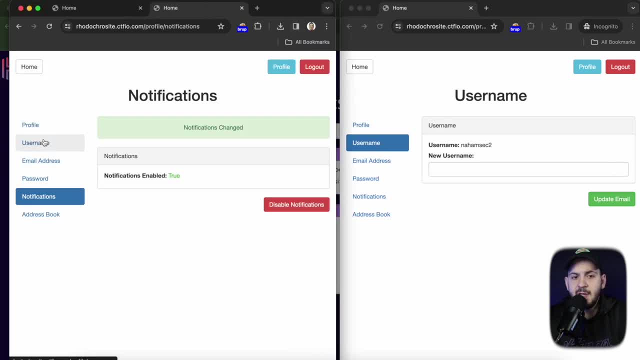 i'm going to perform this action on this other account, so on my build hack secure, which is adam's account, i'm going to make this action, i'm going to call two here and i'm going to intercept. i'm going to take the value for this. 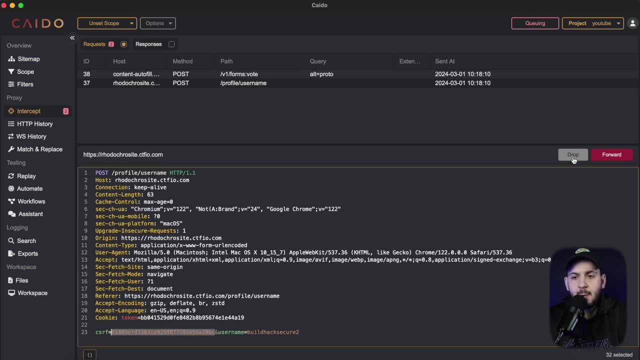 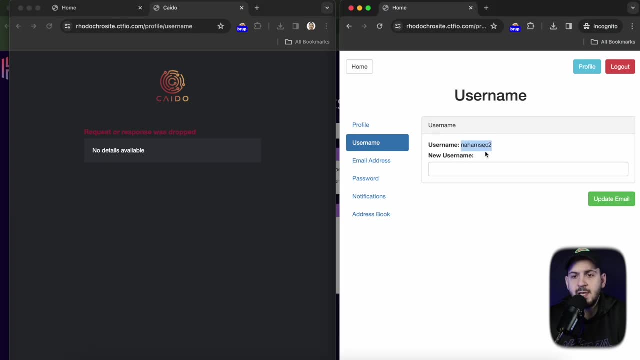 user csrf token and i'm going to drop this request. just in case that you, that value is unique. i'm going to go to my original request for nahamsec. so on this account now we want to change nahamsec2 to nahamsec3, i'm going to replace that token with another user's token, so i have two. 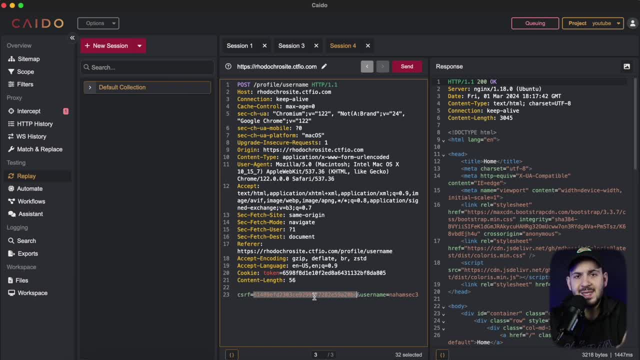 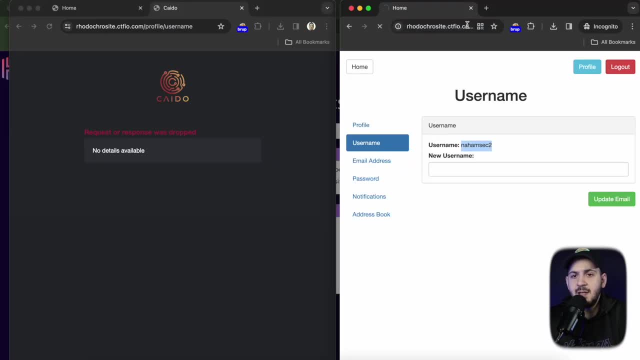 accounts. this one is the one that i want to take over. i perform the action with this account, take its csrf token and put it in here. so if i send this and refresh the page and the username has been changed, it it is going to hint at us that, hey, they actually. 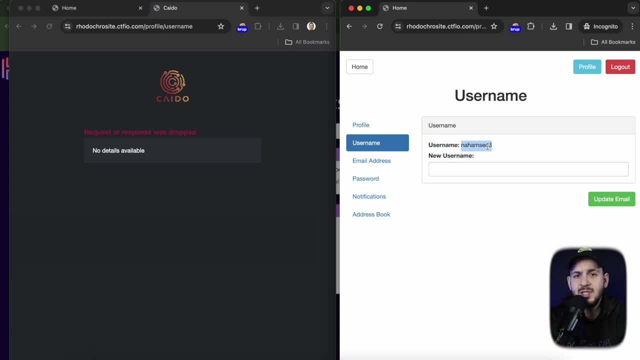 allow you to reuse csrf tokens and the csrf usage is one of the top things i've seen on my pen test and some of these bug bounty programs is that they allow you to do that and by having that bypass you kind of could just do csrf on a lot of different actions. so, and a lot of times i will, 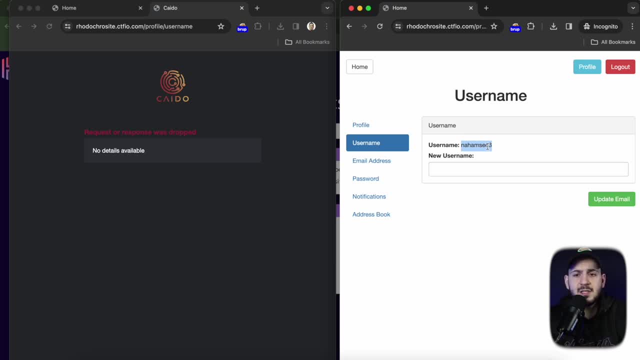 report this as a csrf mechanism bypass. and then if there are some really interesting endpoints, like the email address one, then i would go in there and change the email address to demonstrate a critical csrf where it leads to an account takeover. so if you do see csrf tokens, try to. 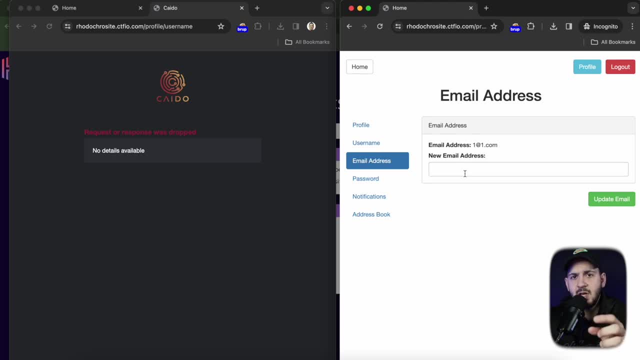 these things, remove them, edit them or also see if you can change the csrf value from account a to account b and see if that request still works. but now let's talk about one more case, a csrf that isn't technically a post request. so for example, in this case, if i saw my intercept again and delete 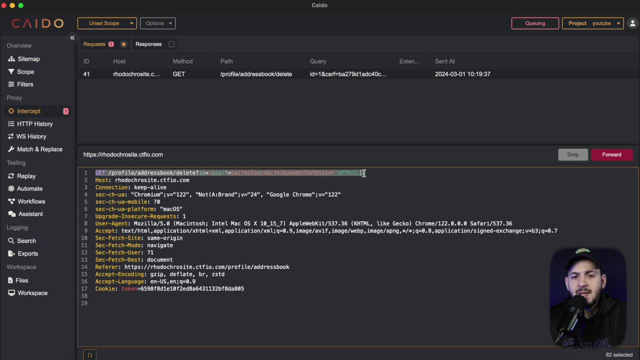 this, we can see that it's actually doing this process with a get request. so in this case, if i send this get request, it is still going to perform this action. so the number one thing we want to try to do is: i want to go in here. i'm going to actually drop this request so it doesn't get deleted. i'm. 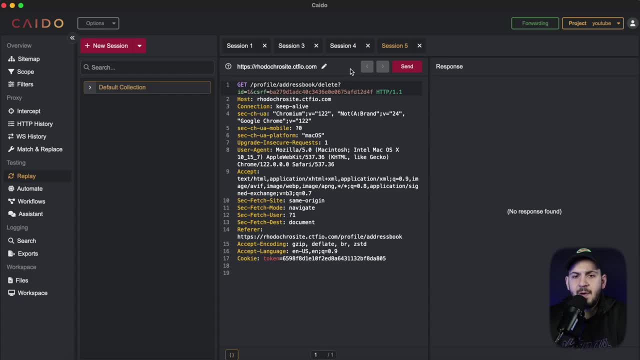 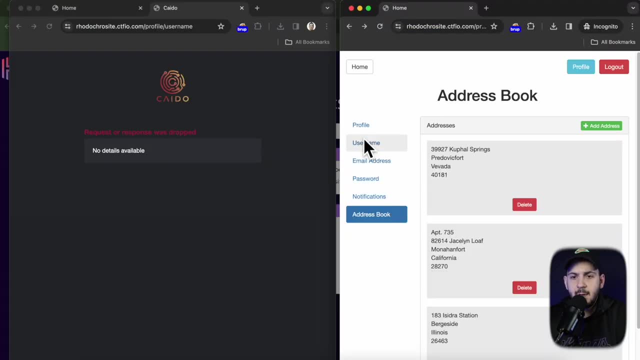 going to go back- our addresses are still here- but i want to see if i can delete this again. i see a csrf token. the first thing i'm going to do is i'm going to send an empty value and if that does work- that didn't work- maybe if i can remove the entire csrf value for it and refresh the page. that one. 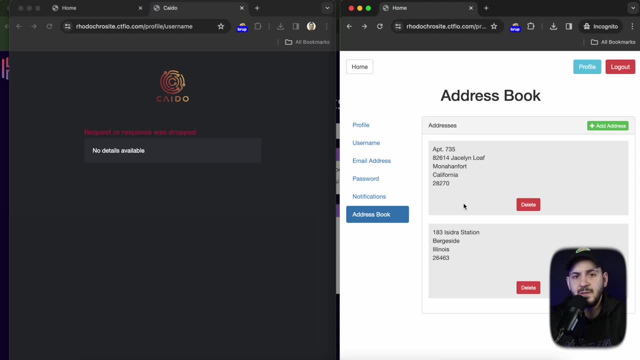 works. so in this case, not only we didn't need to have a secondary csrf token- by removing that entire parameter, it worked- but now what we want to do here is we can actually redo this process. i'm going to actually go into this victim account. i'm going to get my address book. i'm going to get 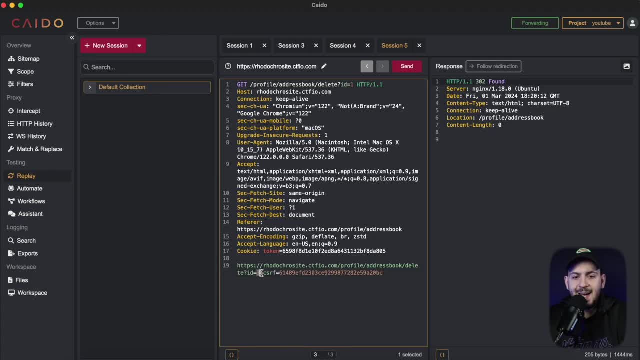 the link for this. drop in here to look at. it looks like id3 is what belongs to that user. so what i'm going to do is i'm going to put that here, id3. and what i'm going to do here is i'm going to make a. 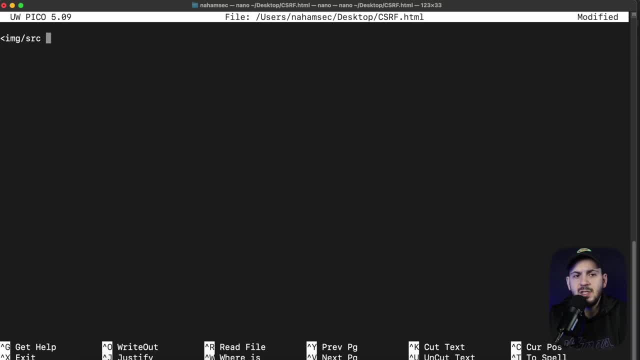 csrf poc. but this one's going to be super easy. you can actually do something like an image tag or an iframe, and then you're going to say: this is the url that i want you to send a request to, and we're going to remove the csrf value entirely.